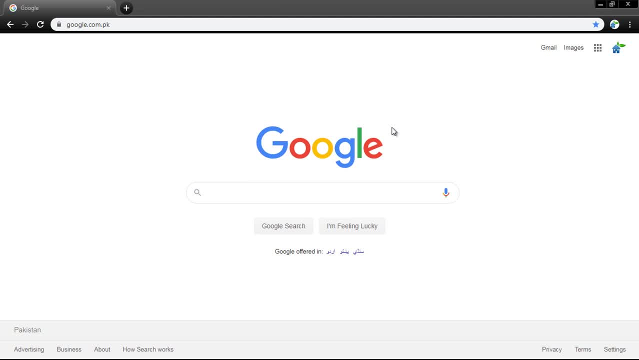 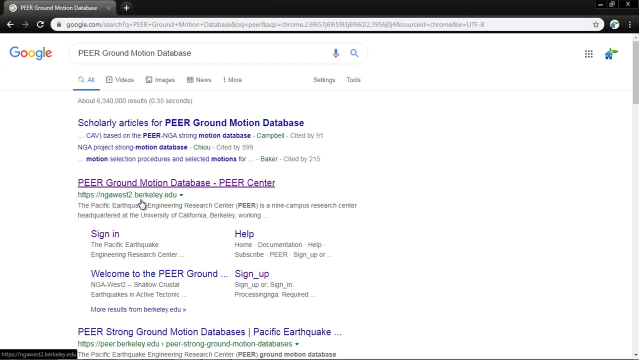 To perform time-history analysis we need earthquake records, ground motion data. To download the ground motion data from the Peer Ground Motion Database and from other sites, here I will write Peer Ground Motion Database. Okay, the first site, that is the ngawest2.budclayedu. that is a site on which all the earthquake records are present. 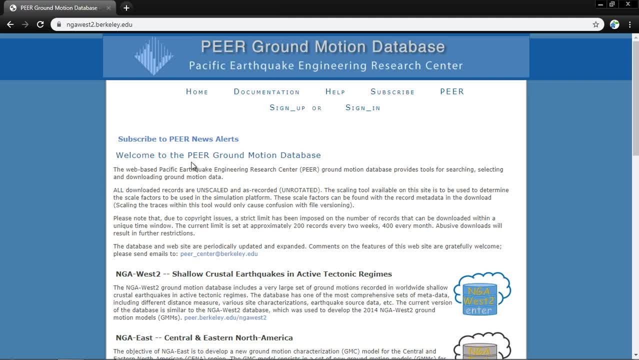 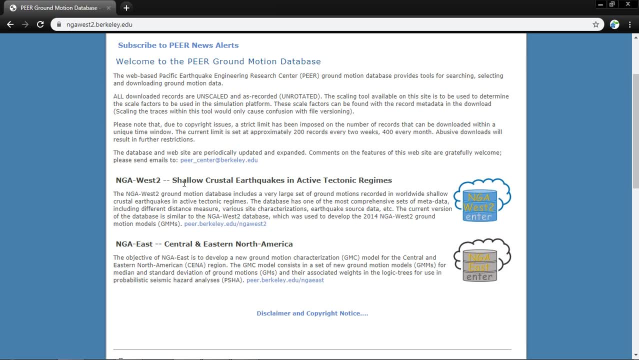 Here. welcome to Peer Ground Motion Database. There are two databases. that is ngawest2.shallowcrustearthquickinactivetechnology In active tectonic regimes, that is a nga west and that is a nga east. In the nga west all the records- worldwide shallow crustal earthquakes in active tectonic regimes, all the earthquake records and the central and eastern North America records are in the nga east. 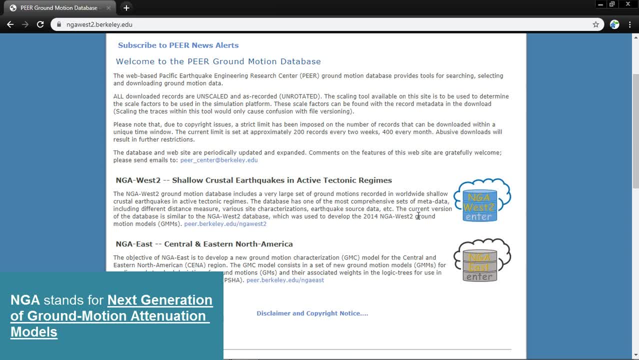 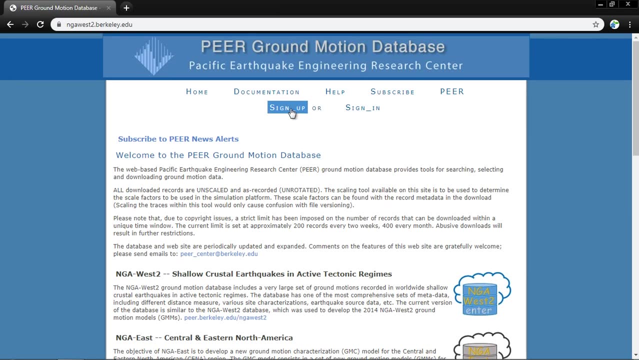 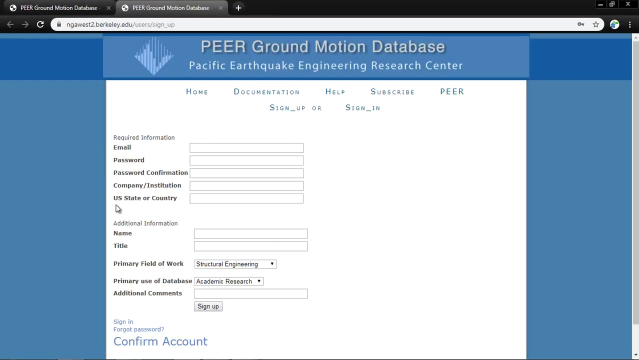 So for the worldwide, for almost all types of data like imperial, Kobe, Taiwan, smart, all types of North America records are in the nga east, Northridge Newhall. all types of earthquake records are present in nga west2.. Okay, so you have to make sign up. For sign up you need email address, password, all types of things. Any student of university or any commercial person can download these data records and these are freely available by Peer Ground Motion Database. 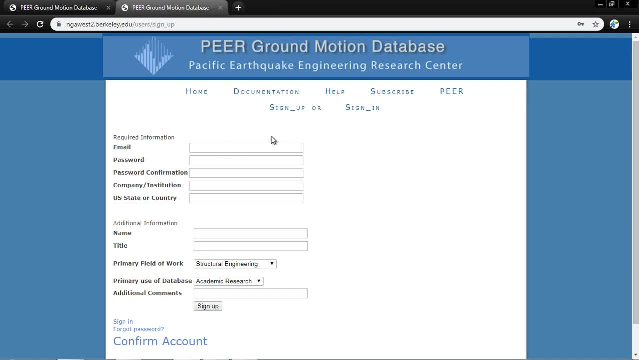 So I have already made the sign up. First of all, when you make the sign up, then they will send you confirmation mail and you will confirm. then you can come back and sign in Here. I am going to sign in. 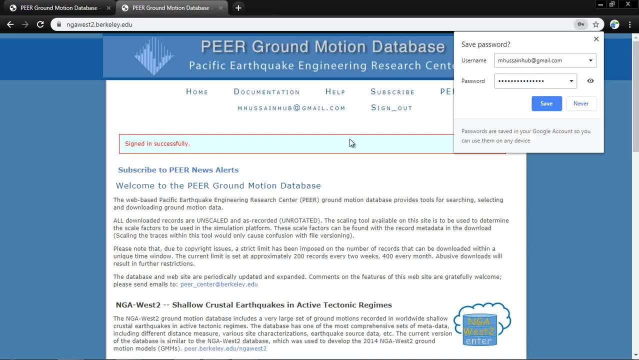 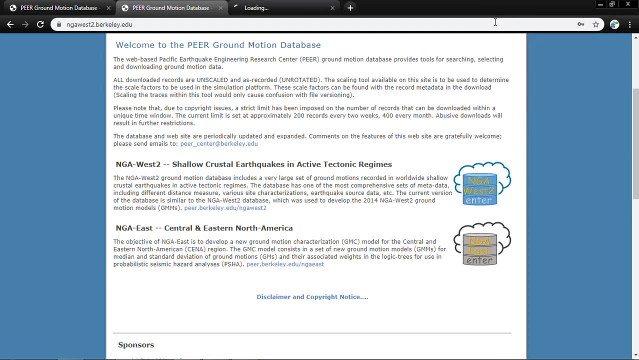 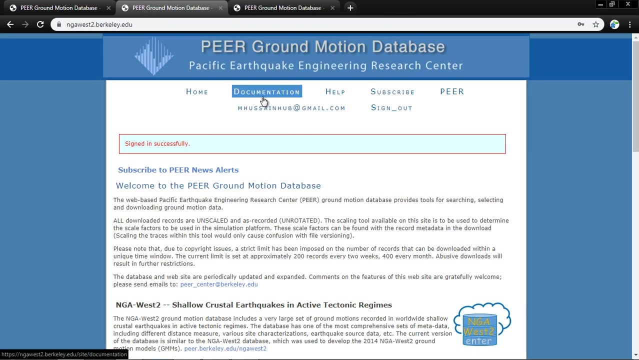 Sign in. Okay now, Now I am sign in successfully. Here is mhusainhub at gmailcom. Now I will click right click and open in new tab nga west2 database. So this site will open and on this main site you will click documentation. 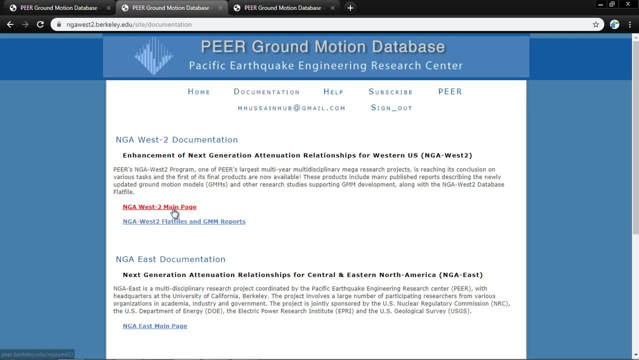 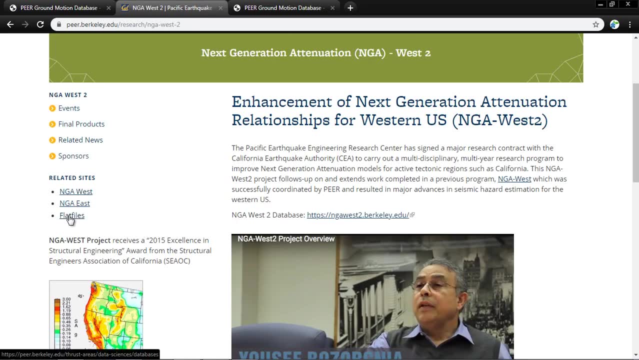 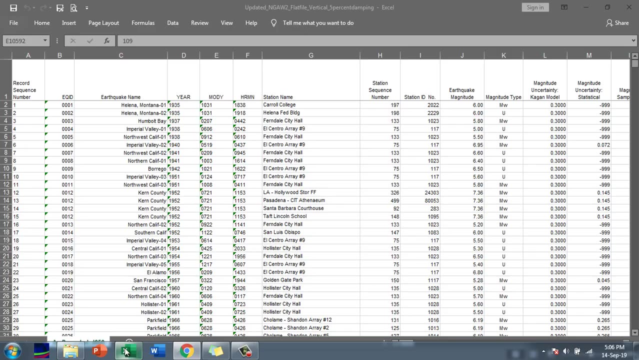 In the documentation you will click nga west2- main page. In the main page here you will click flat files. In the flat files the record of all earthquakes are present in the excel sheet. So here you can see record of all around about 21,000 earthquakes. 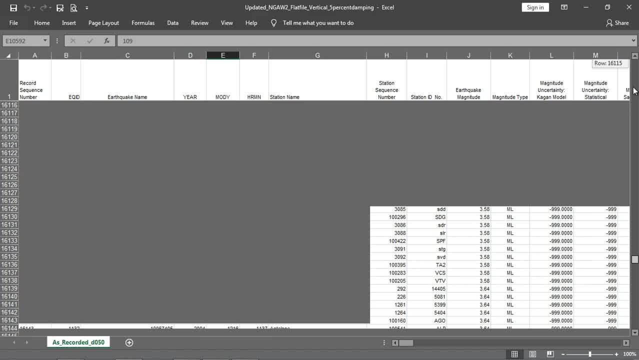 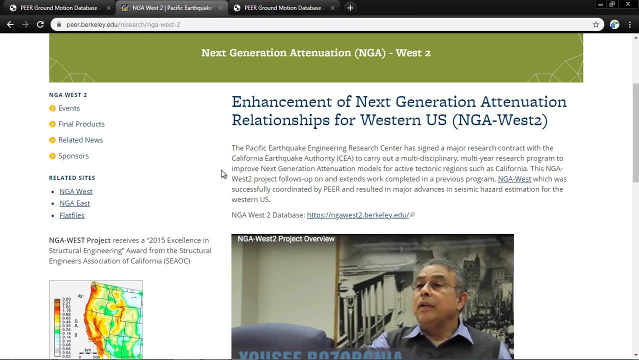 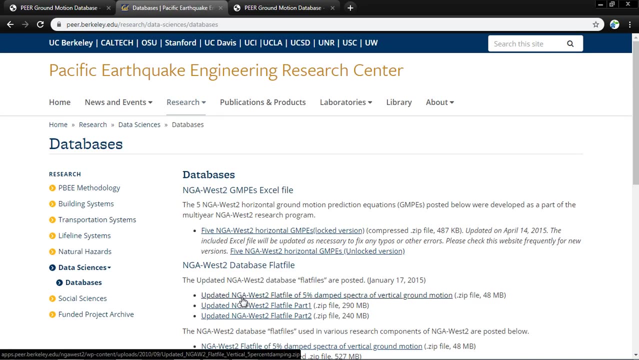 Okay, earthquake records are present. Okay, in this one file, that is a flat file by Peer Ground Motion Database. Here you will click flat files. Here you will download updated nga west2 flat file of 5% dam spectra of vertical ground motion. 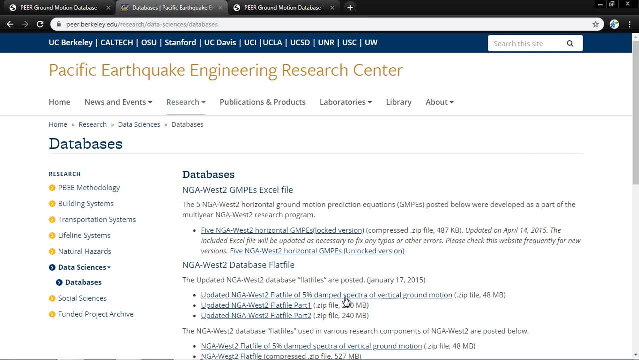 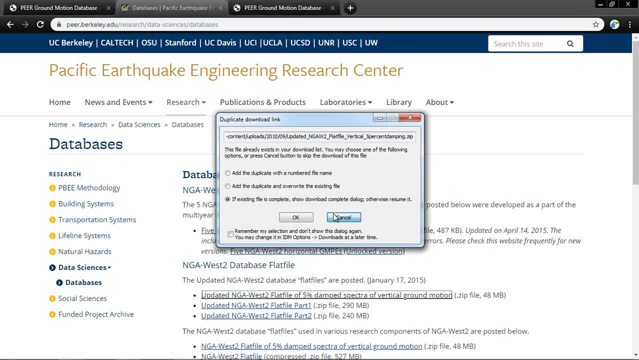 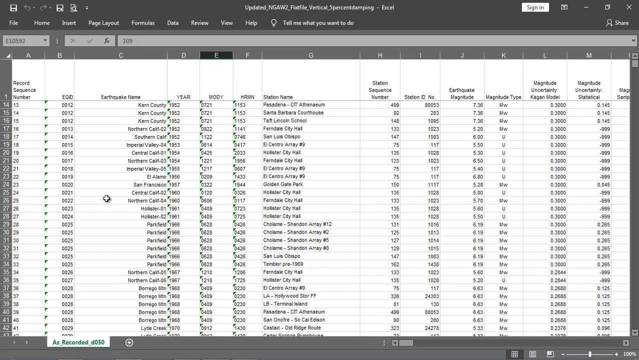 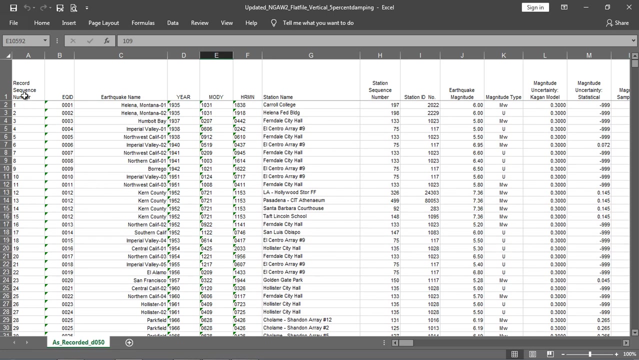 So here, when you will click, because I have already downloaded and after downloading I have unzipped the file because that is a zip file, and here is the downloaded file. In this all records are present, For example, record sequence number, RSN number, earthquake ID, earthquake name, year. 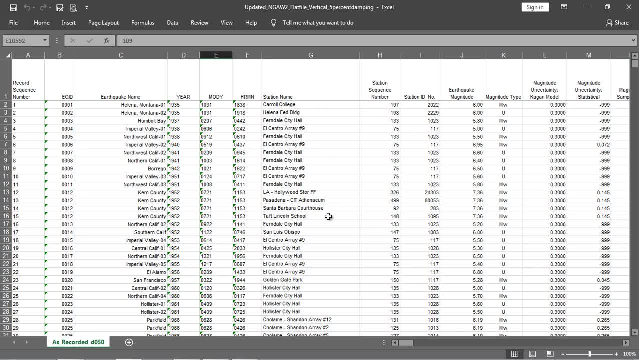 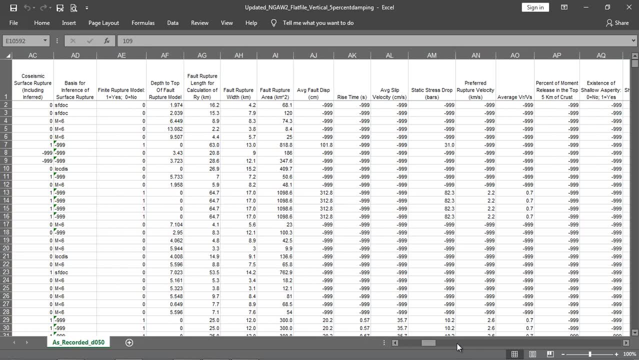 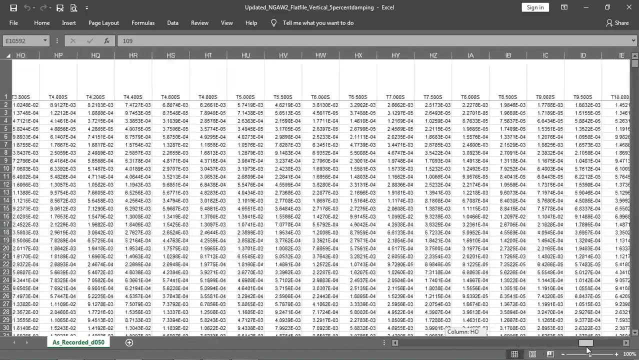 Okay, and station name: earthquake station. this is located. earthquake magnitude Okay. soil type. all types of data which is required by the researchers. Okay, all the property data are present. Now I will show you how you can download any database. 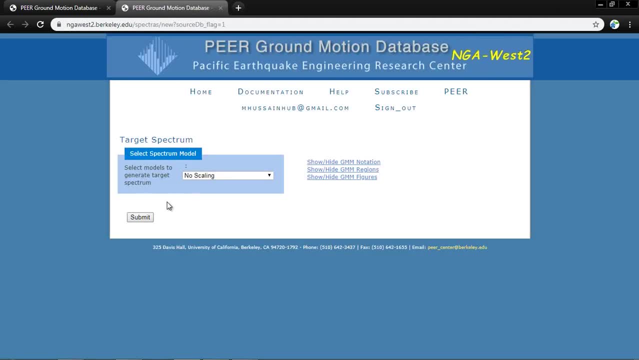 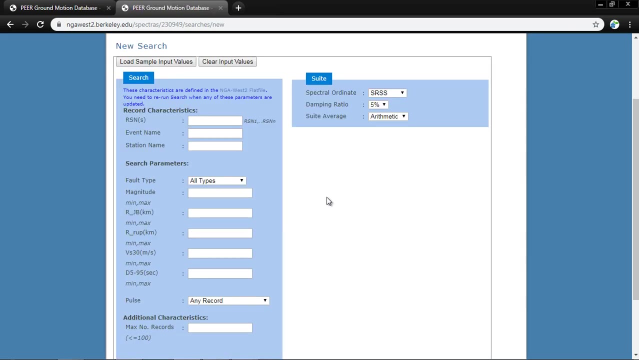 Now I will close this file. You will click after coming to this page from this right click and come to this page. please press submit. Okay, now there are two ways for the searching of any earthquake. For example you will. here is the load sample value. 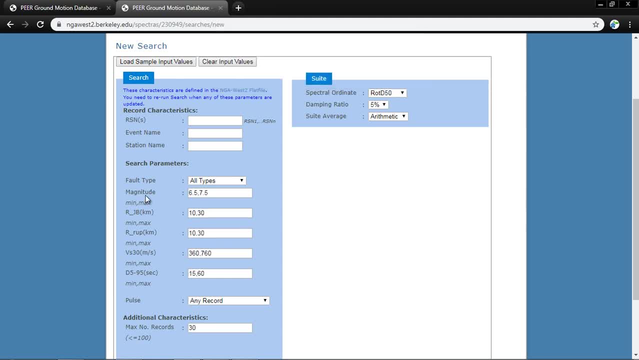 Okay, are you sure? Yes, I want the magnitude of earthquake 6.5 to 7.5.. For example, I need to earthquake record from 5.5 to 7.5, or maybe 6 to 7.5.. 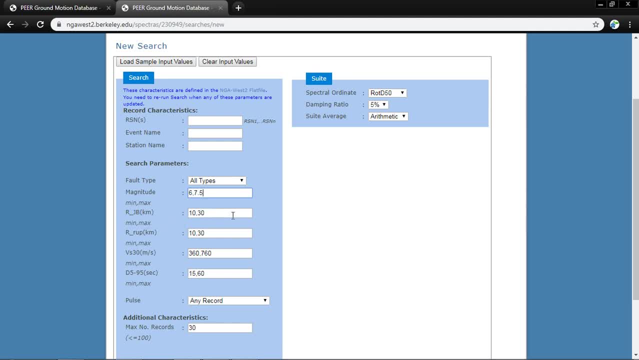 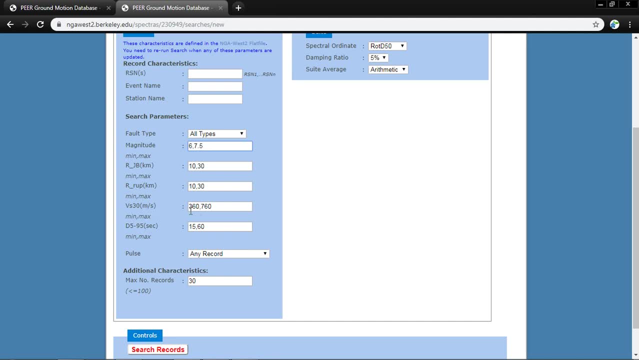 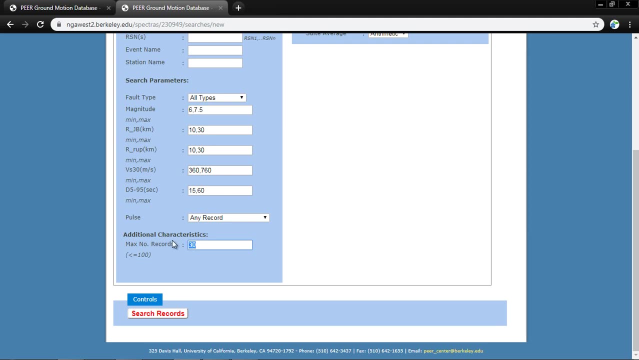 RGB in kilometer 30 to 30, 10 to 30 kilometer range, R rupture in 10 to 30,. shear wave velocity: 30,, that is, 360 to 760.. Okay, so all types of data For example I want to record, maybe up to 90.. 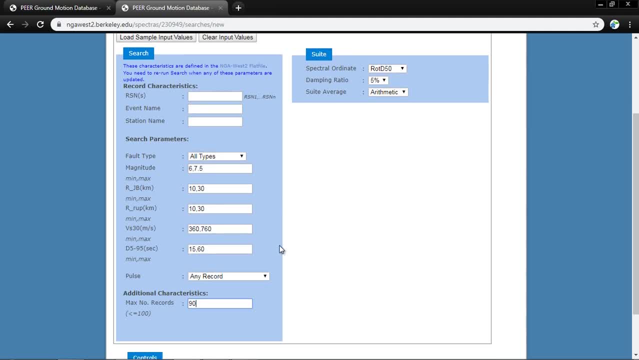 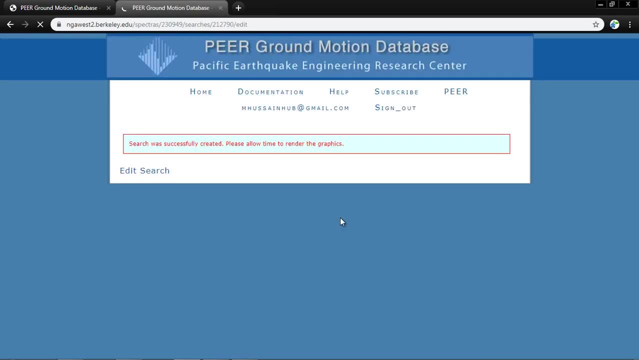 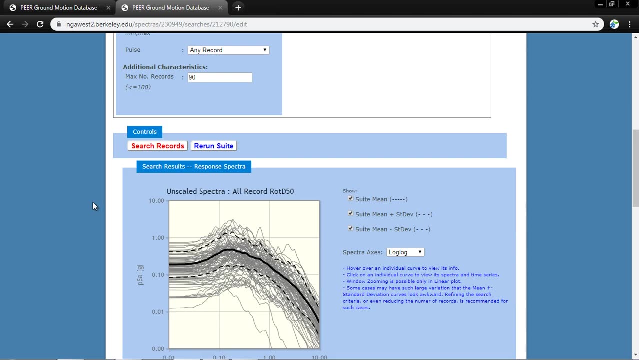 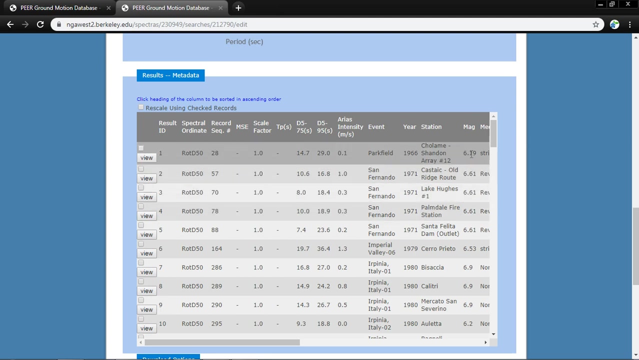 When you will put your desired values and then search records. Okay, software will give you all the search results, all the results here. Now you can see the magnitude here: 6.19, 6 point. you can see increasing values all the up to 7.. 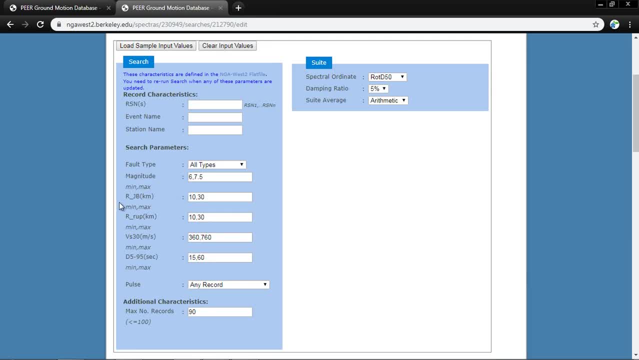 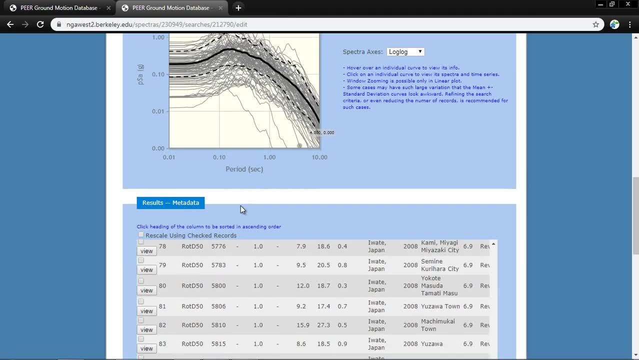 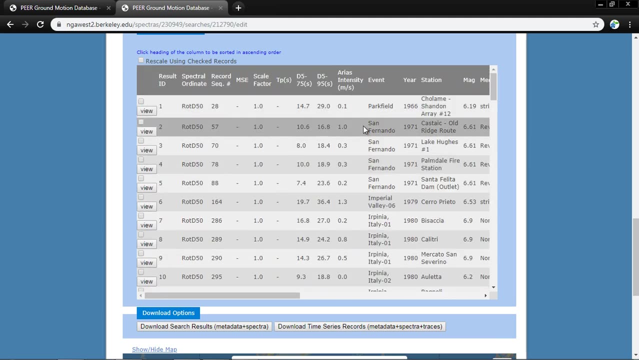 The range I have defined in the magnitude, all types of filters. after applying all types of filters of peer ground motion database, given these earthquake records, You can see any record, Okay. So, for example, let's see this first earthquake, Okay. 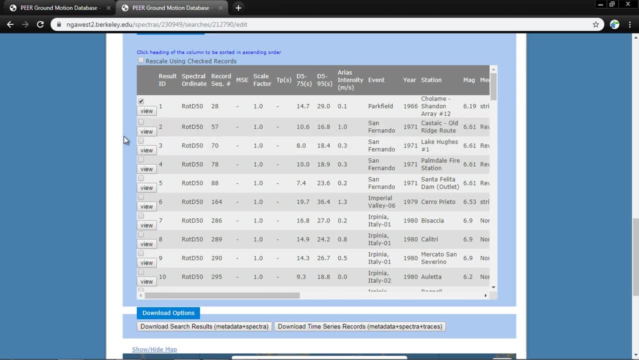 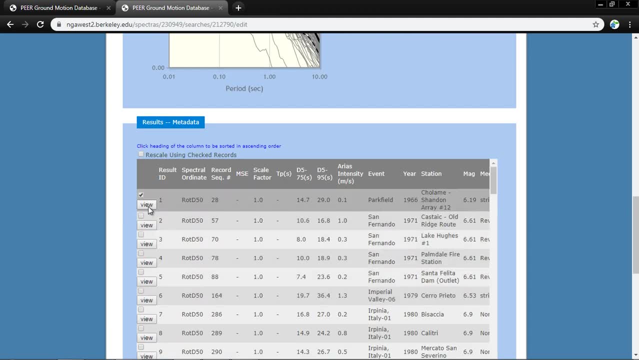 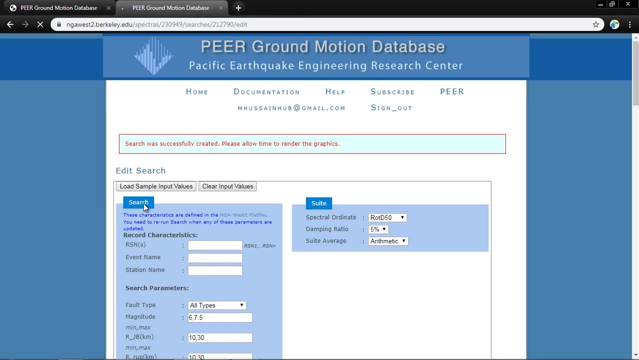 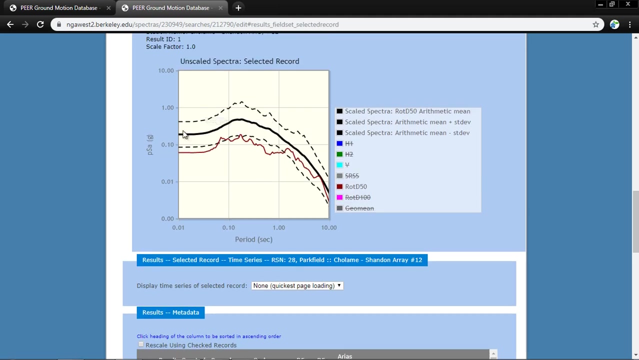 Click here and press view. And this is the basically response of all the records which the software had displayed downward. Now I will see only one, The card of only one. Okay, here you can see the card of only one file scale spectra. 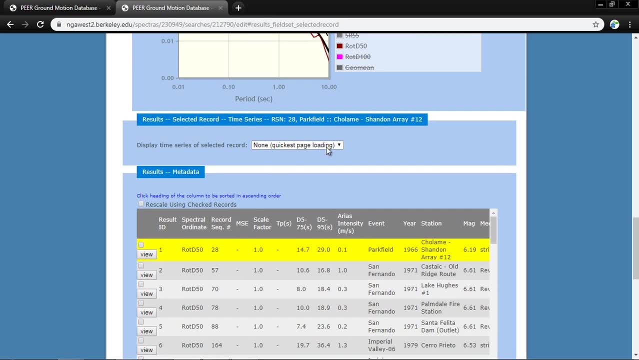 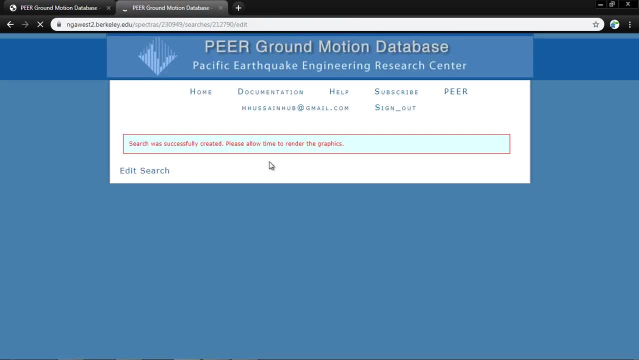 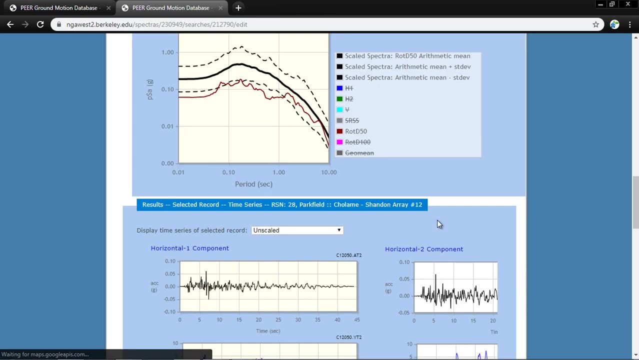 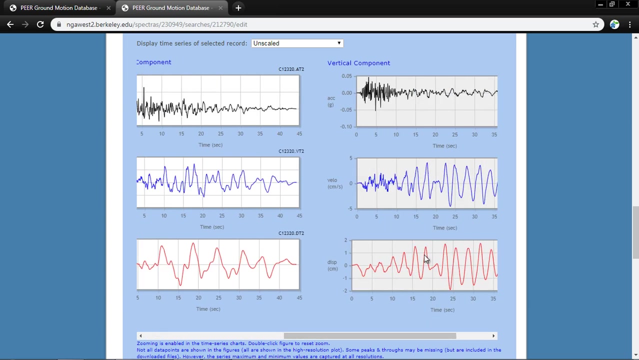 Okay, so now I want to see its time history called. So just click on scale. Okay, here is the time history called horizontal component one, horizontal component two, And here is a vertical component, And the first one is in acceleration. 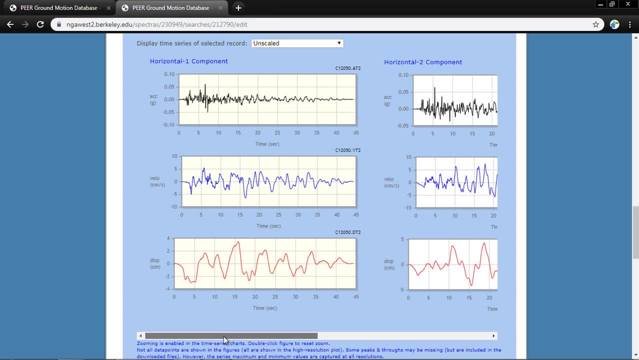 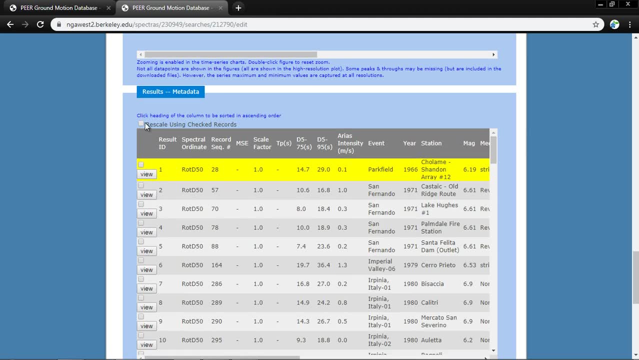 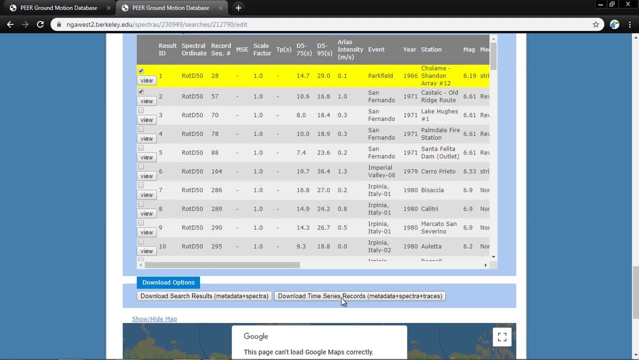 The second was in velocity. Third, one is in displacement. Okay, And after that you can also select all records And then just press download All the records means acceleration, velocity and displacement, And if you want to download only spectrum, so you will click here. 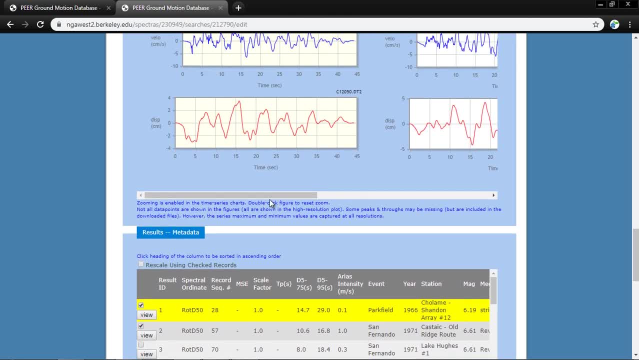 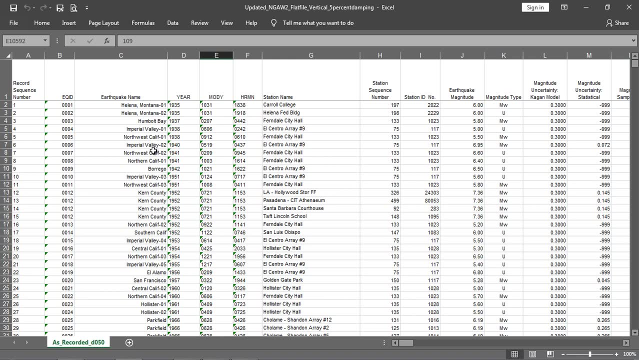 Okay, I will download and show you also. So now, what is in this flat file? For example, I want the imperial valley, Sorry. Now I want imperial valley, 1940 earthquake record. So that is a very famous earthquake record which is used by the researchers. 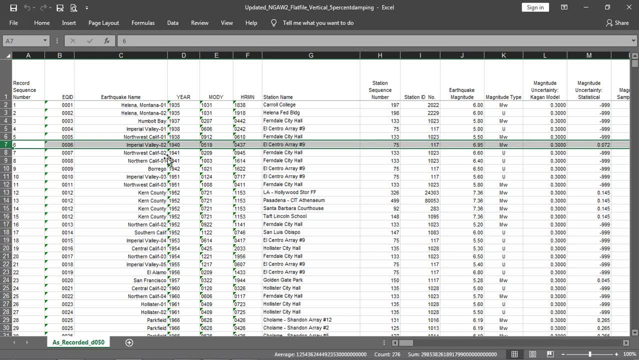 If you study research papers you will see almost in every paper imperial valley earthquake. So the earthquake record which is used, almost its second name- is Alcentro earthquake also, So that is in 1940.. So how I can download? I have to just note down this RSN number, record sequence number. 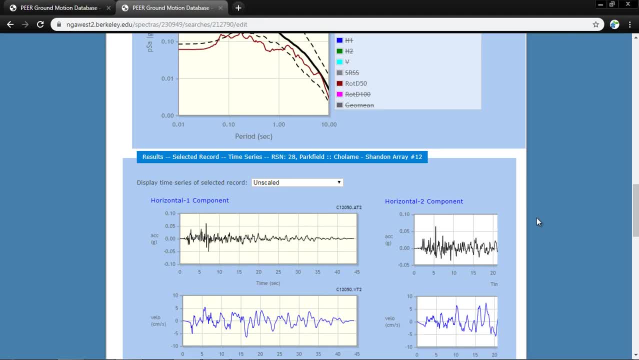 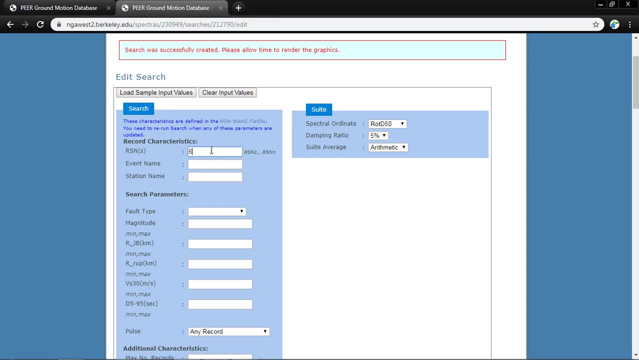 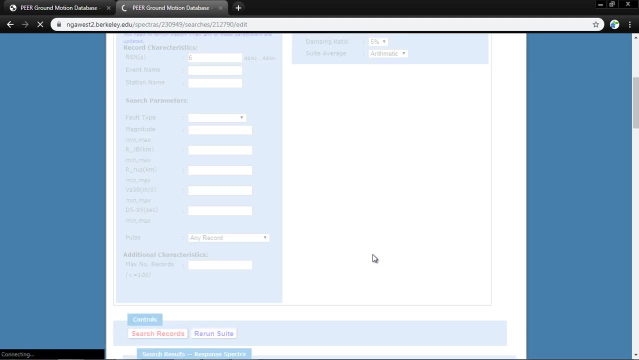 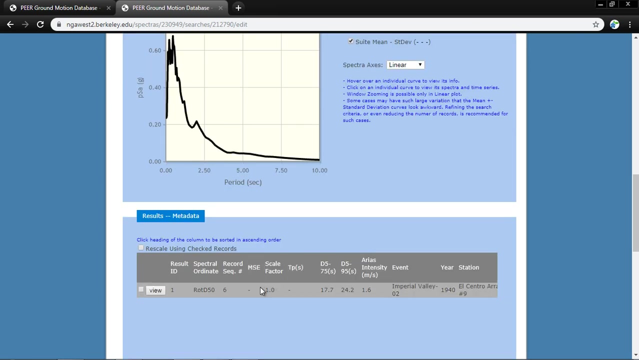 That is six. Okay, Now I will go up Clear input values. Okay, Now I want to download the required sequence. number six, That is imperial value. Now I will click search records. Okay, When I will come down. here is a imperial valley: 02 1940 earthquake record: Alcentro array. 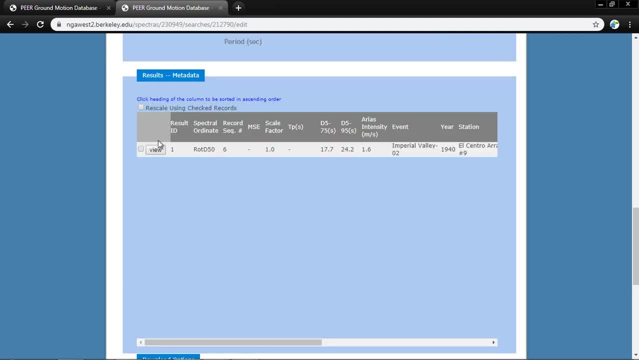 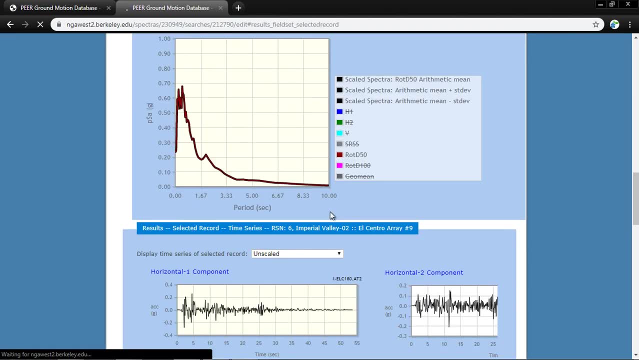 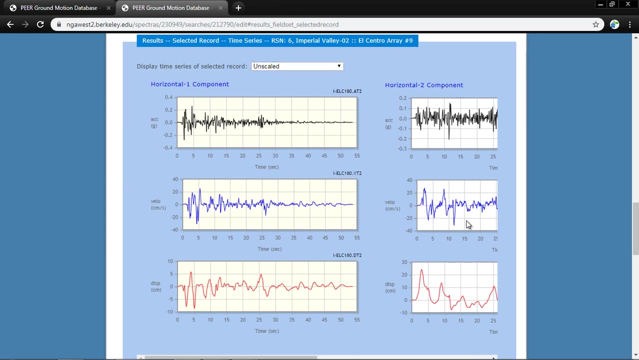 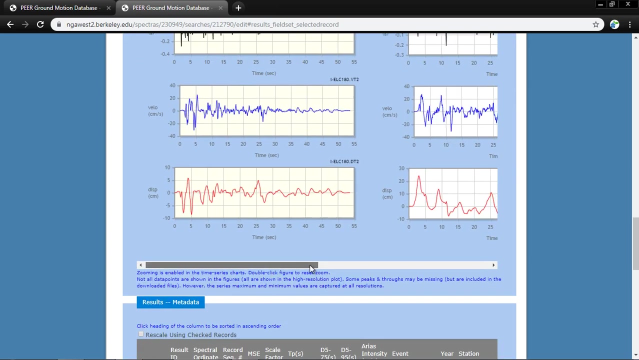 So all the values are here. Okay, So now I will also view. Okay, Here you can see the unscaled. You have to select this unscaled, Then these records will display. This is a horizontal component: acceleration. horizontal component. second: horizontal component: vertical component. third: 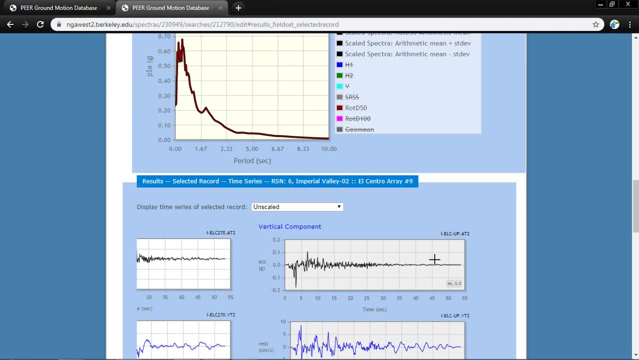 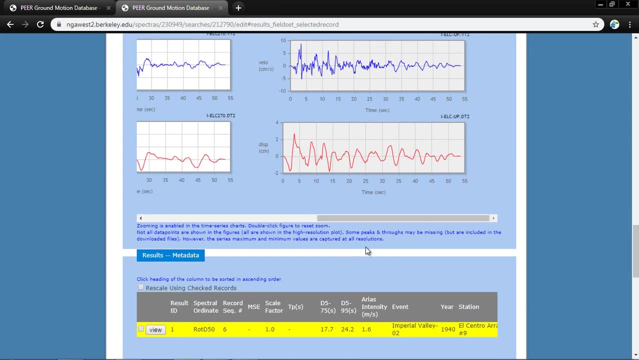 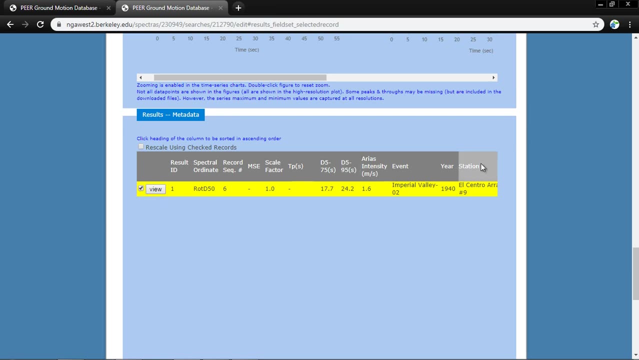 Each earthquake have three components: horizontal X, horizontal Y and vertical. Okay, That may be at any angle, Okay, So here I will download these nine files. Okay, For downloading all these nine files I have to select, Then click here. download time series records. 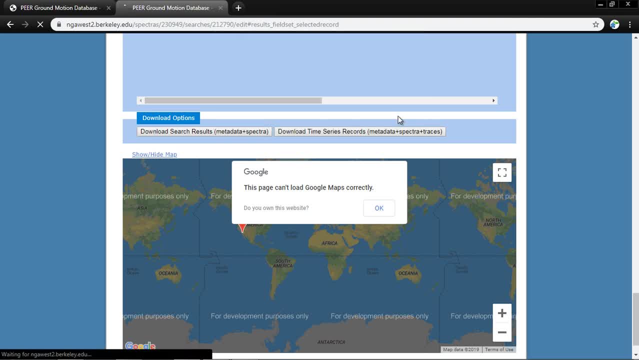 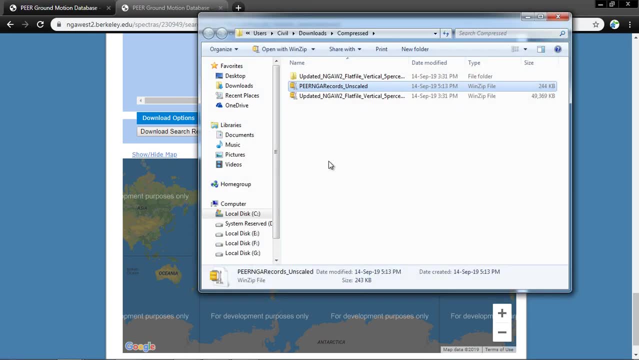 Okay, Okay, Okay, Start downloading. Okay, When the software download. Now I will just extract these records. Okay, Here, all the all nine files. Here there is. you will see the symbol AT2, DT2 and VT2.. 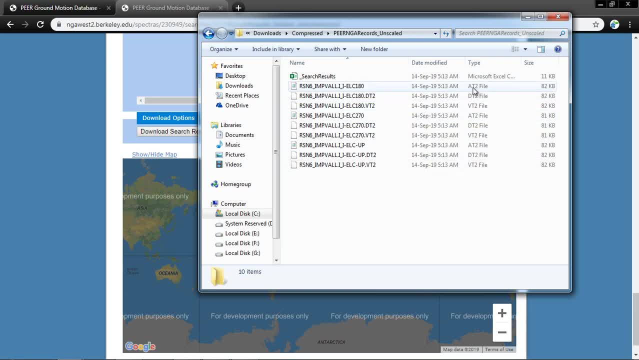 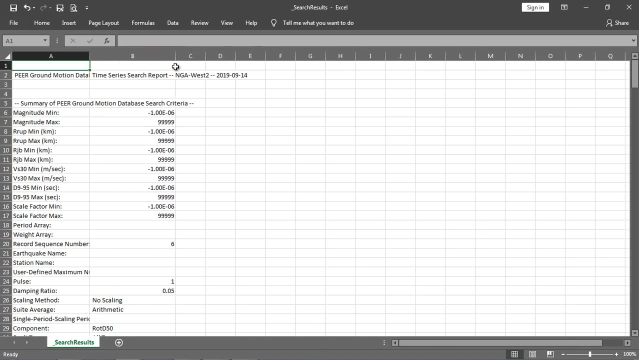 Then that will repeat What is our. A is for acceleration files, D for displacement files, V for velocity files. In the search results you can also see the nomenclature. Okay, Here the file name extension mean acceleration, velocity, displacement. 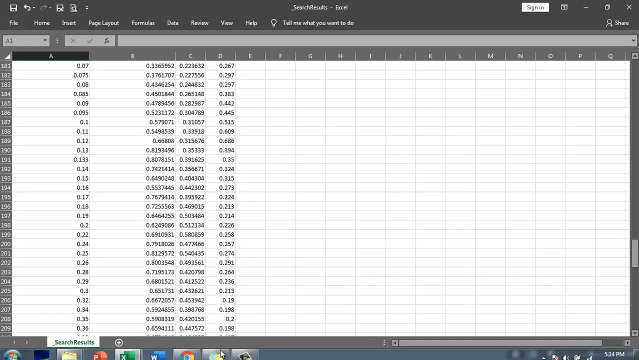 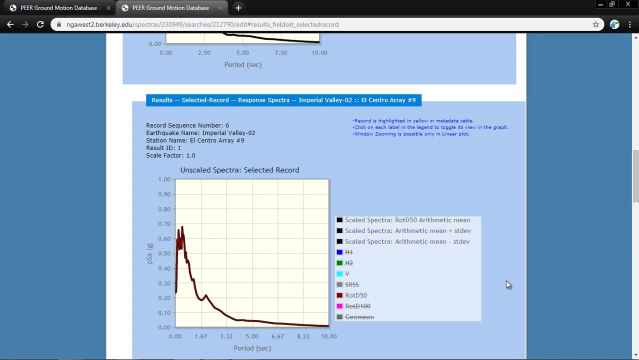 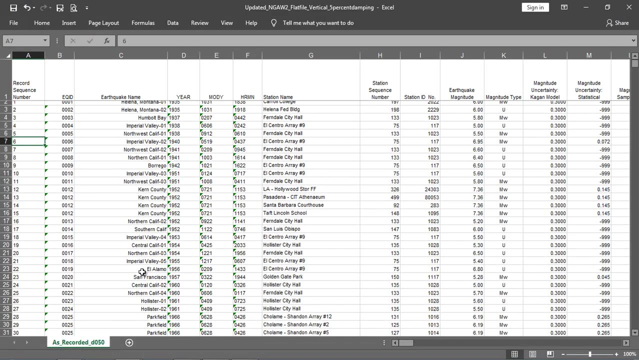 Here the response spectrum files. Okay, The files which software is showing here? Response spectrum files. Okay, You can also study. Here is the data record. Now I will do the second example By using, for example, Kobe earthquake. 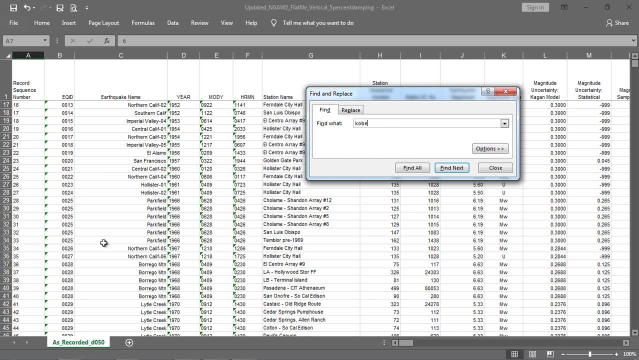 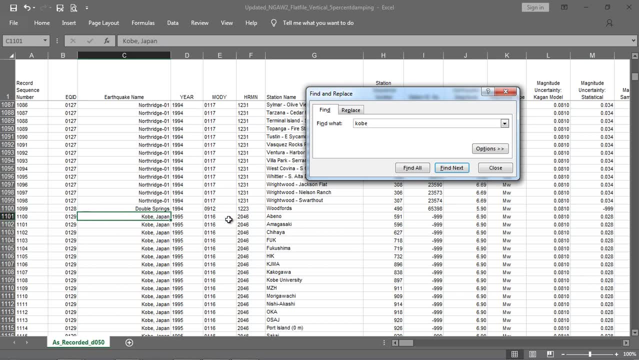 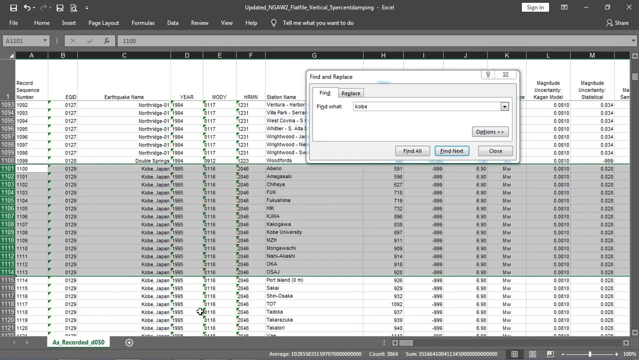 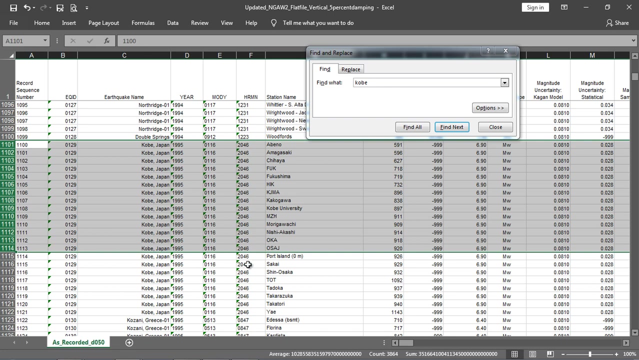 Control F Kobe. Okay, That's a Kobe, Japan earthquake. So here is a Kobe earthquake. Kobe earthquake is recorded at different stations- Okay, Here. So now I will download Kobe, For example. Let's suppose I want to download the Kobe University record here. 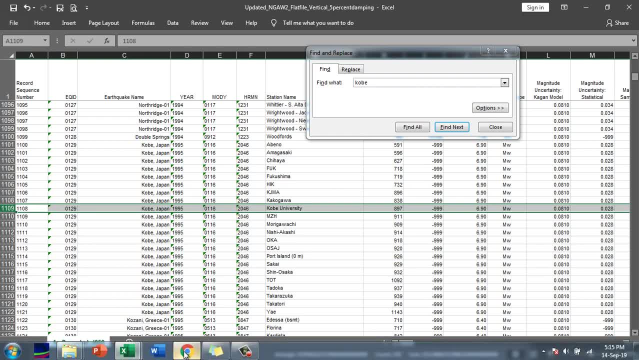 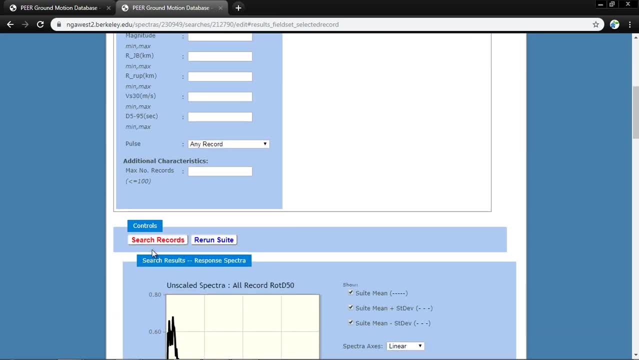 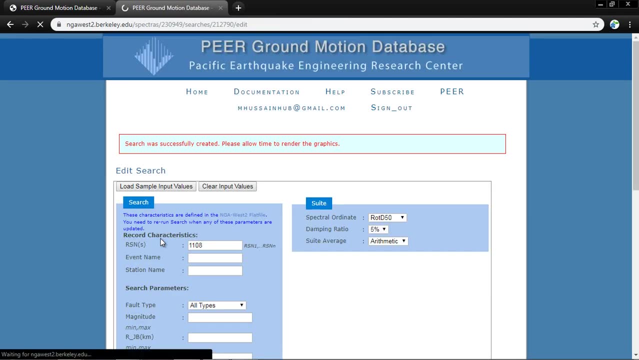 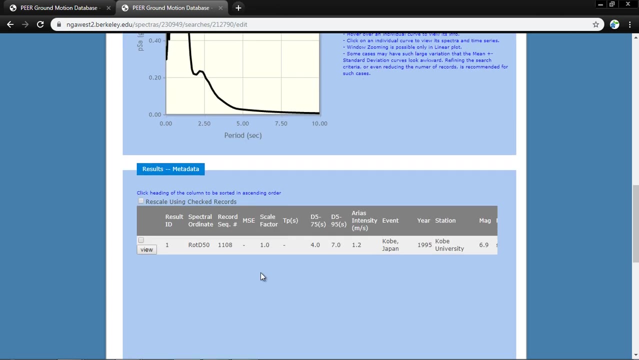 It's record sequence number is 1108.. You have to just put that value: 1108.. Okay, Now here, search record. Okay, Search record. And then here is the record. Okay, If you want to view again. 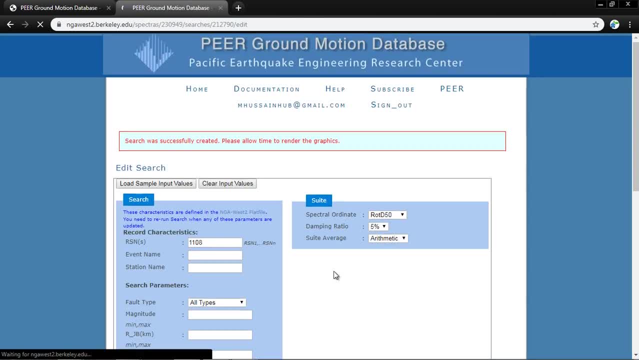 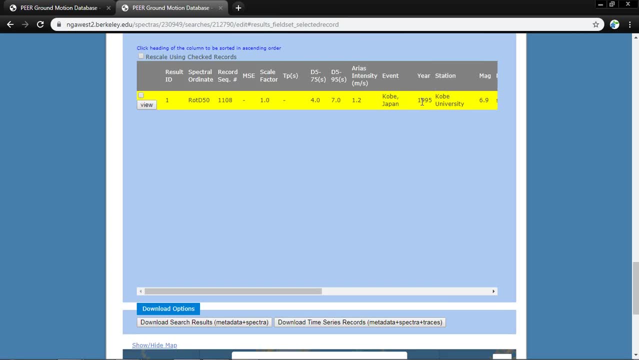 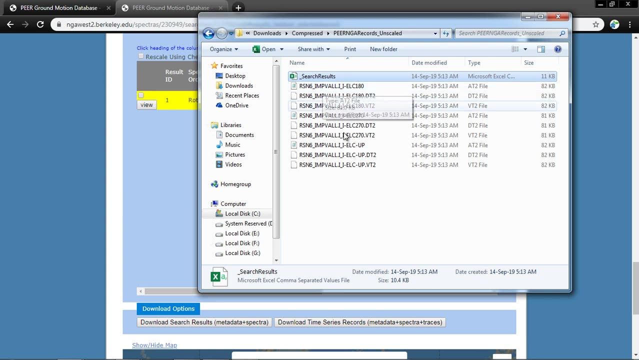 You can view. Then again you can download the record data. Here all the files Again you can download: Kobe University 1995.. Kobe, Japan. Okay, So here you can also view the file. Here is three files, One is at 180 angle. 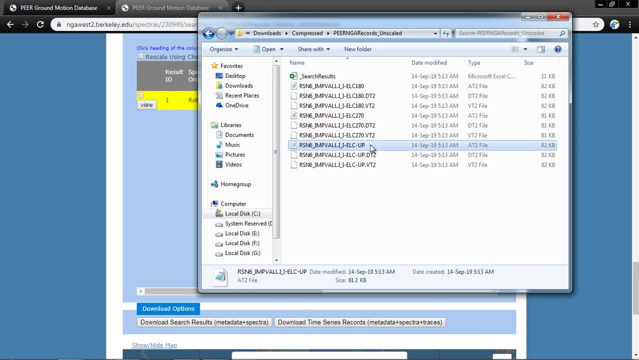 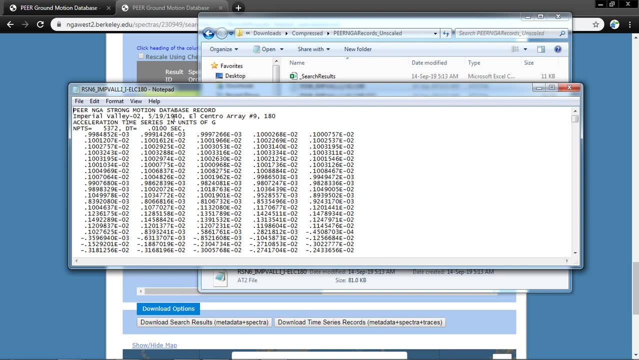 Second, one is 270 angle And one is up, So here I am clicking Peer NGA strong motion database, Imperial Valley. That is earthquake recorded All central array station. Okay, That is the angle Acceleration times. All the values are in G. 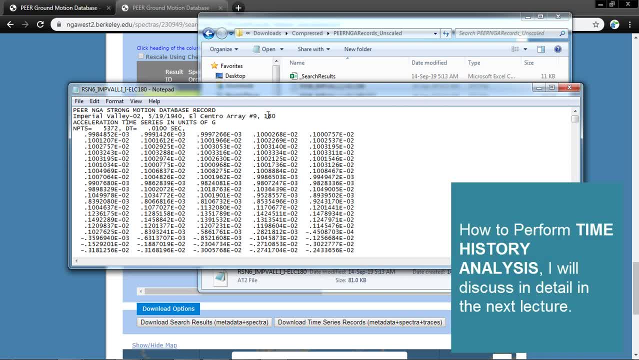 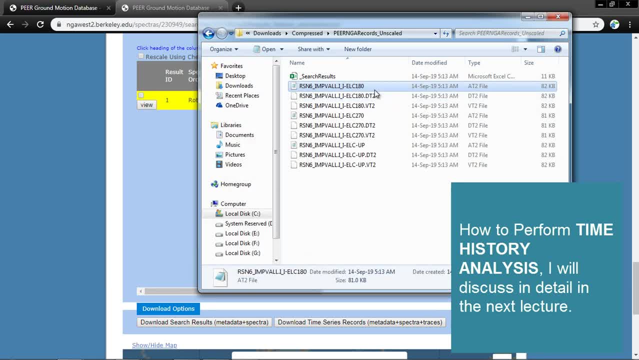 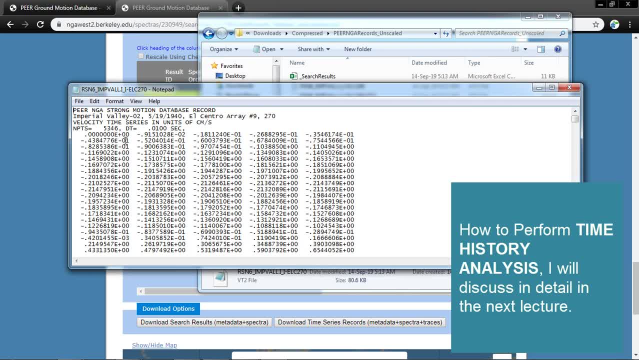 You have to right click Open, Select a program. Here you have to select notepad, Okay, Then you will see all these values. Okay, database. have a nice day.